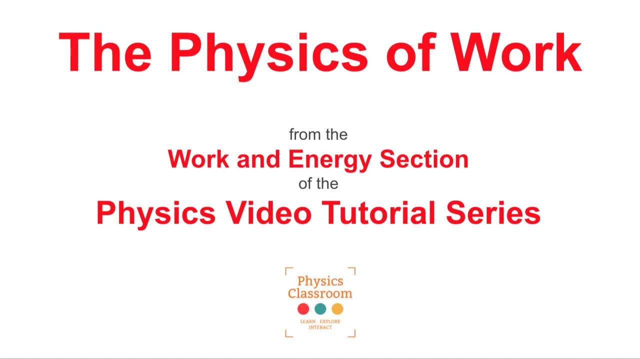 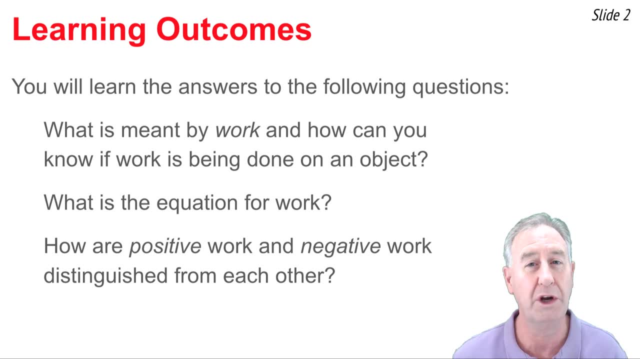 Welcome to the Physics Classroom's video tutorial on work and energy. The topic of this video is the physics of work, and we want to know, first, what is meant by work and how do you know if work is being done on an object. Second, what is the equation for work And third, how are positive 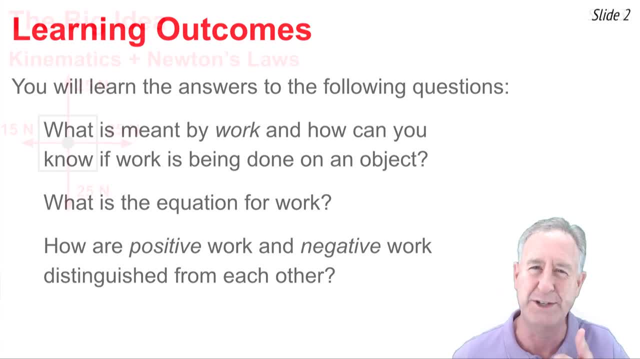 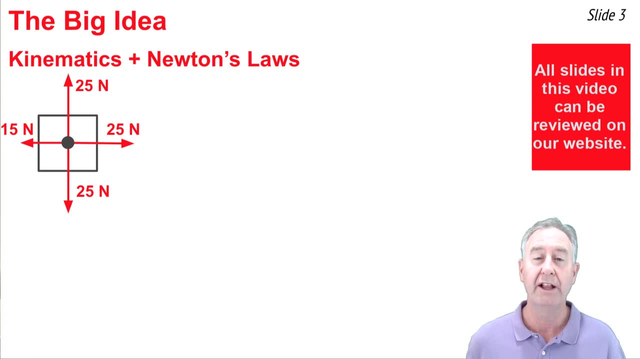 and negative work distinguished from one another. I'm Mr H. Let's get started. This is our first video in our tutorial series on work and energy. Before we begin talking about work, let's talk about where we're going with this tutorial series. In previous video tutorial, 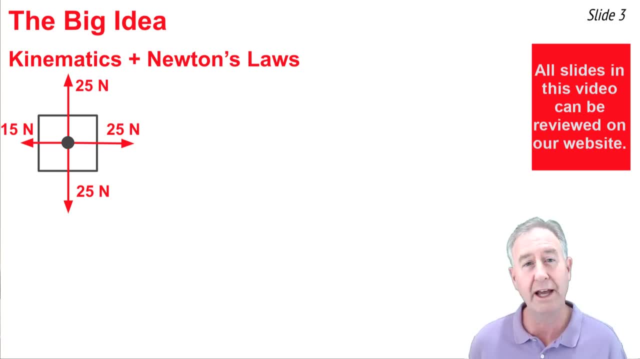 series we've talked about Newton's laws and kinematics, And one of the big ideas of those two models combined is that we can use Newton's laws to determine the acceleration of the object. We look at the forces that act upon the object, We determine the net force and find the acceleration. 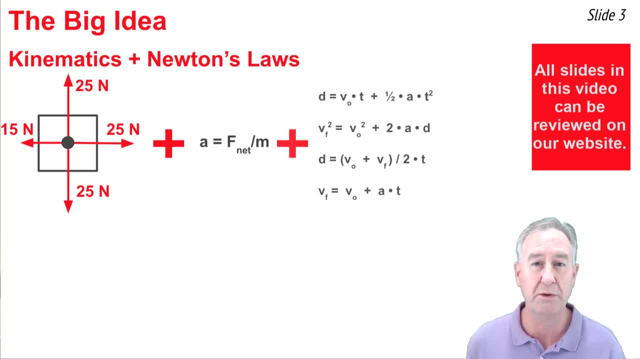 This acceleration is related to things like the distance the object would travel or how fast the object would be moving. We have a series of kinematics equations that help us relate acceleration to things like distance, final velocity, initial velocity and time. We can use 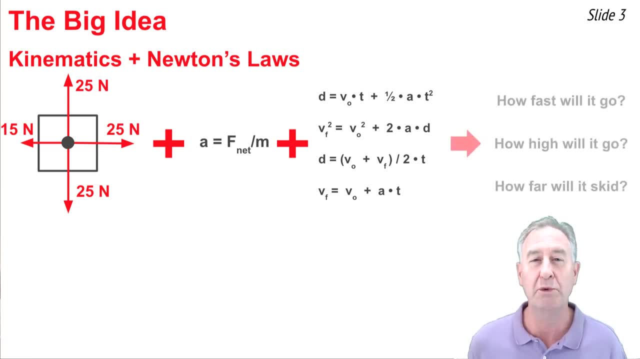 these two models. in order to determine how fast an object will be going, how high it will go and how far it will skid Along the way, we may introduce several representations like velocity time graphs, position time graphs and dot diagrams In the work and energy model. 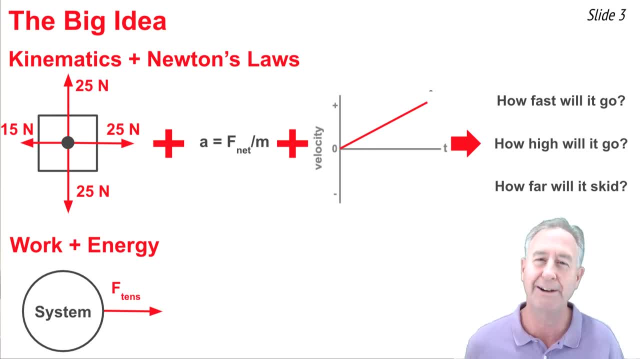 we attempt to answer the same types of questions, but do it in a different way. We imagine that object or collection of objects being a part of the system. We look at the forces that act upon the object. We look at the forces that act upon the object. 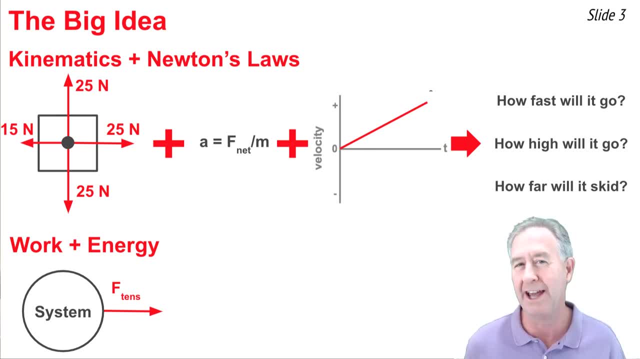 And we look at the forces that act upon the object. And we look at the forces that act upon the object. We look at: how does the system interact with the surroundings? what forces act upon that system, that object or collection of objects? We do this in order to determine what is happening to the 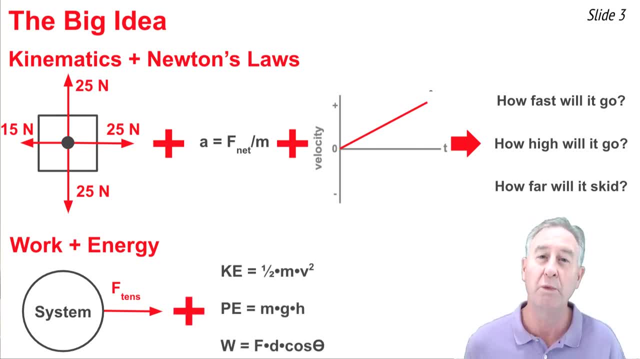 kinetic or potential energy of the object, so that we can predict: will the speed increase or decrease, will the height increase or decrease or will these remain the same? And finally, we want to determine the answers to questions like how fast will it go? how high will it go? 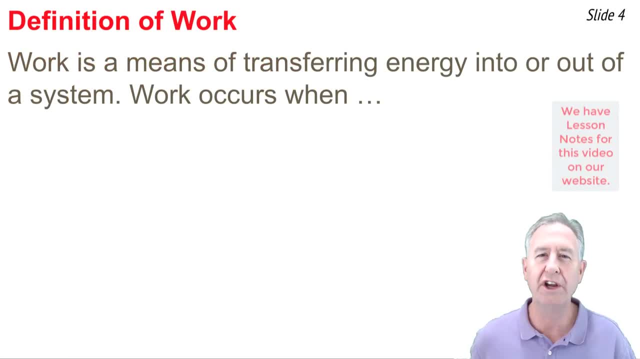 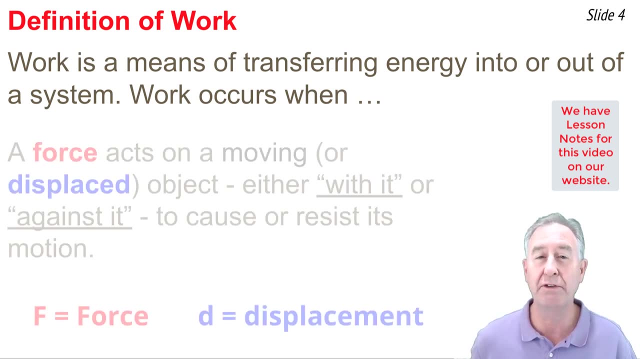 and how far will it skid? In physics, work is considered a means of transferring the energy of the object. We look at the forces that act upon the object And we icit experience this variation. by transferring energy to or out of an object, Work occurs. 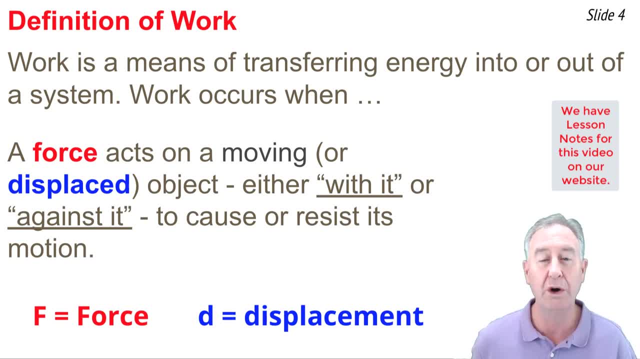 whenever there is a force acting upon a moving or displaced object, That force could be with the object's motion or against the object's motion, That is, in the same direction that the object is moving, or in the opposite direction that the object is moving. When considering, 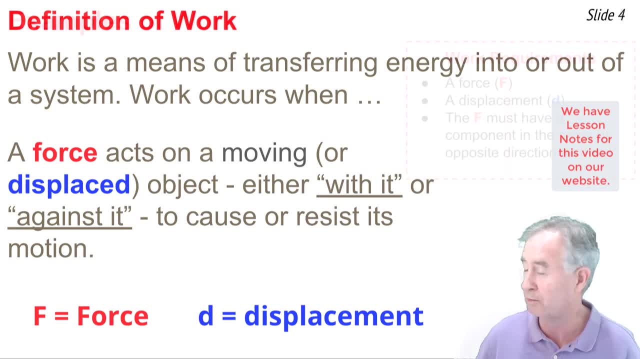 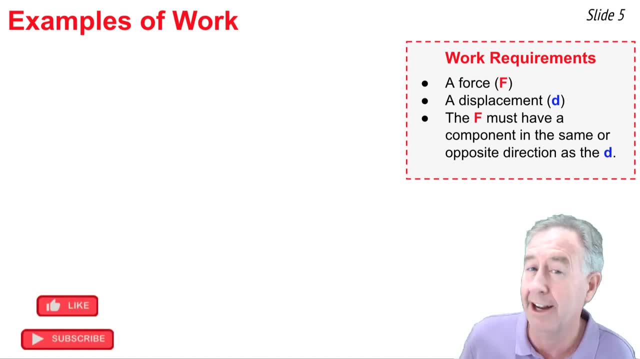 work, we have to think about two big ideas: force and displacement. Let's talk about some examples of work, But before we do, let's requirements. there must be a force acting upon the object and the object must move or be displaced, and there must be some component of the force or part. 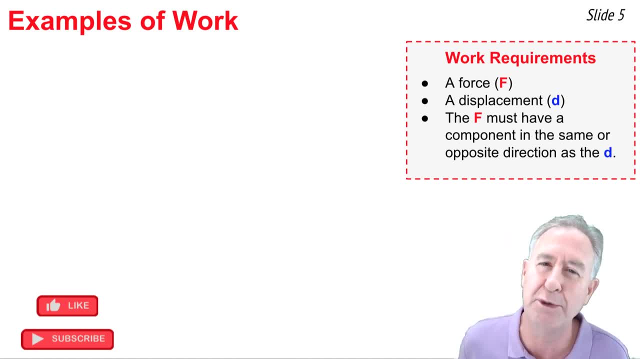 of it that's directed either in the same direction or the opposite direction as the displacement. so let's consider: two students push on an out-of-gas car in order to move it towards a gas pump. here we have work being done on the car. there's a force acting on the car. the students are pushing on it and the car 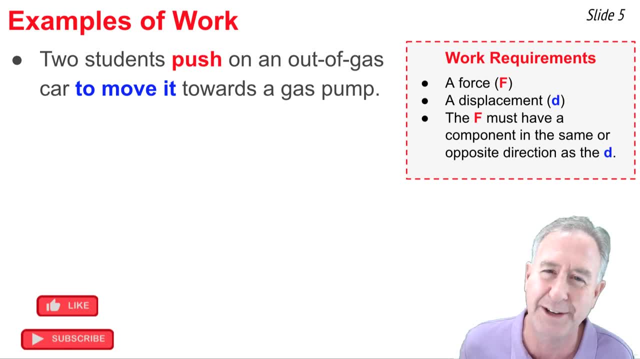 is moving and the force is in the same direction that the car is moving. in our second example, let's consider a freshman exerts a force on a world civilization book in order to lift it up to the top shelf of this locker. in this case, there's work being done on the book, the student is pushing on it and the book is. 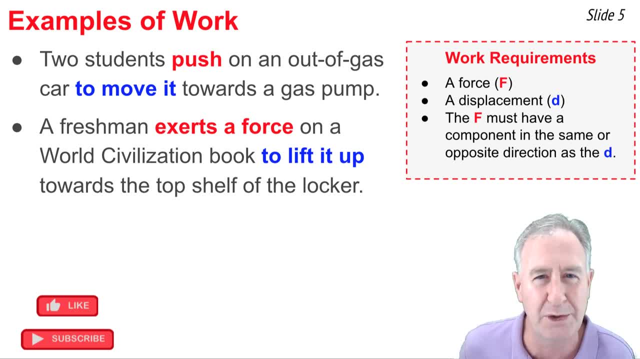 moving. the student pushes up to move the book upwards. that's work. in our third example, let's consider a book that has been nudged off a table and free falls and accelerates towards the top of the book, towards the ground. this is work being done on the book. there's a force of 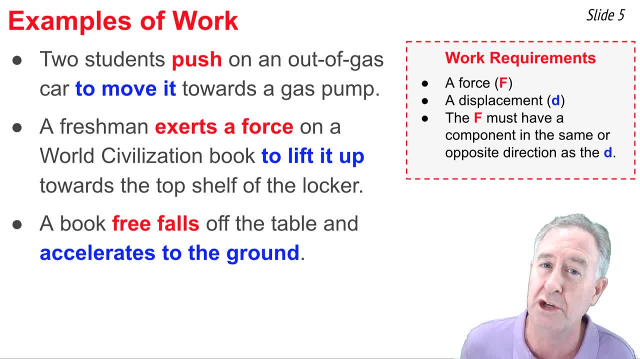 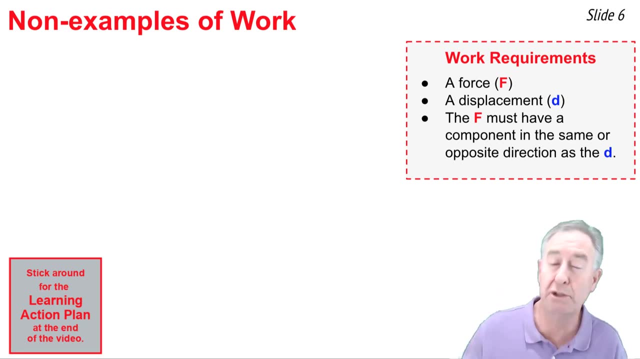 gravity acting on the book and it acts in the same direction that the book is displaced downwards. that's an example of work. in all these examples we have a force that acts upon an object to cause the objects displacement. now let's consider some non examples of work in light of these three requirements of. 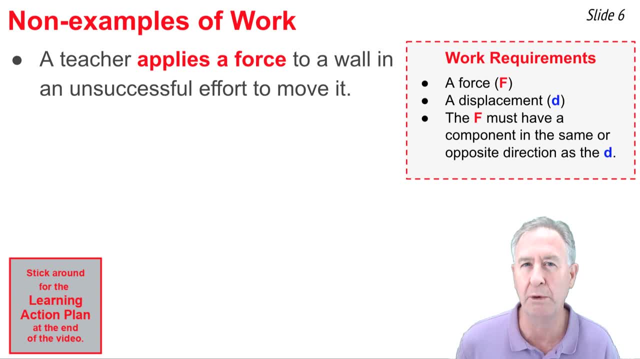 work. in the first situation, a teacher is pushing up on a wall, becoming totally exhausted in an unsuccessful effort to move the wall. in this situation, there's a force on the wall, but the wall is not moving, and so it doesn't meet the three requirements of work. there's no work. 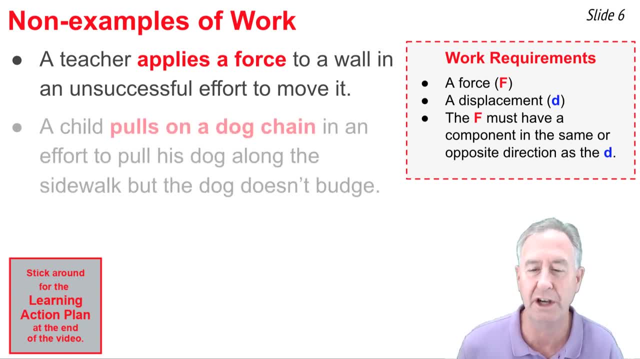 done on the wall. in the second situation, a child pulls on a dog chain in an effort to pull the dog along the sidewalk, but the dog just doesn't budge. in this case there's a force on the dog, there's a tension force, but the dog 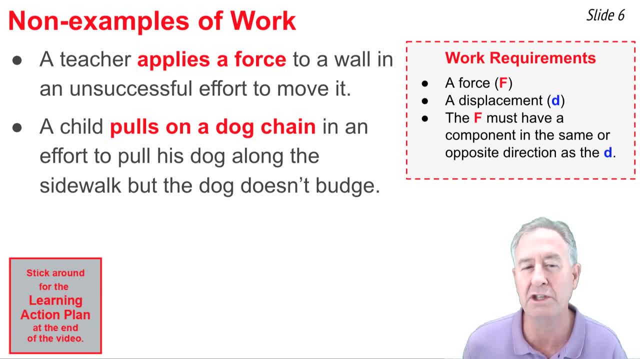 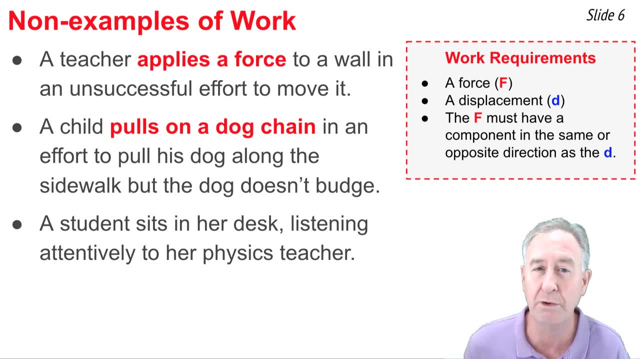 doesn't move, there's no work done on the dog. in our third situation, a student sits in her desk listening attentively to her physics teacher, who wouldn't a hundred dollars. in this situation there's a force upon the system, abnormal force, hop in a gravity force down, but the student doesn't move. it's. 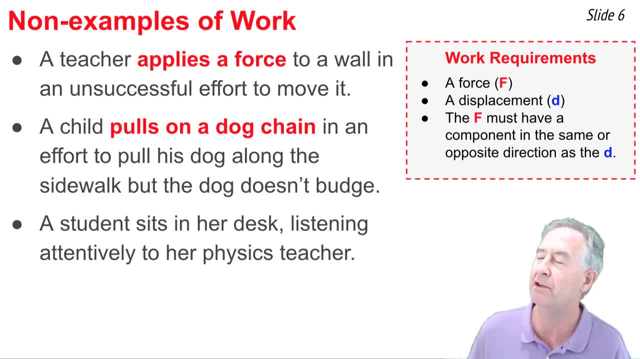 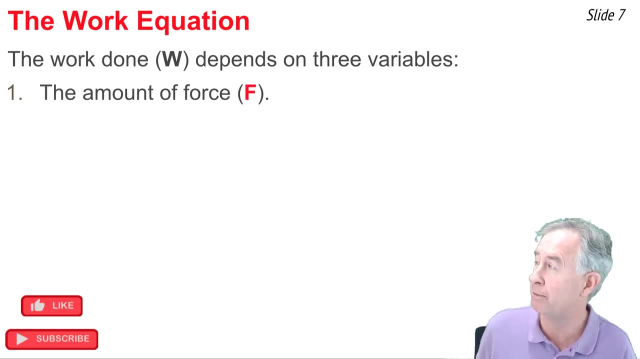 not displaced, and so there's no work done on the student. in all three examples we have situations in which there's a force but no displacement, and so there's no work done on these objects. mathematically, the amount of work done upon an object depends upon three variables. it depends upon the amount of: 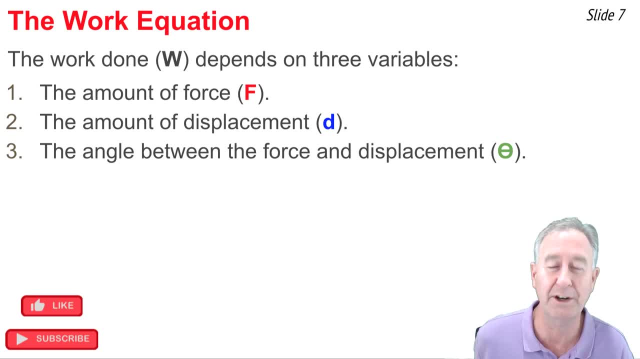 force, the amount of displacement and the, the force vector and the displacement vector. We can express these dependencies with the equation: work W, equal force, F times displacement, D times the cosine of the angle between the force and the displacement vectors. The unit for work is the joule, abbreviated J. One joule is equal to: 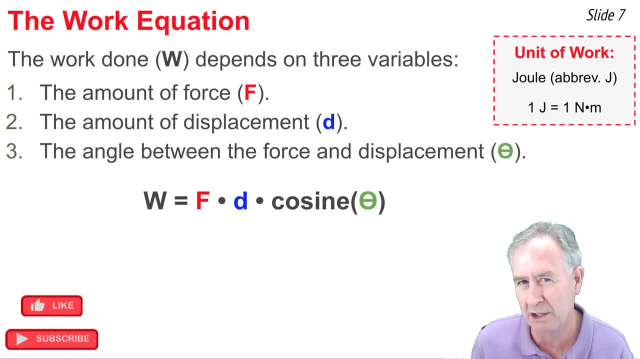 one newton times one meter, as inferred by this equation. The most complicated part of the equation is the angle, theta. Theta is the angle between the force vector and the displacement vector. If these two vectors are in the same direction, then theta is zero degrees. If they 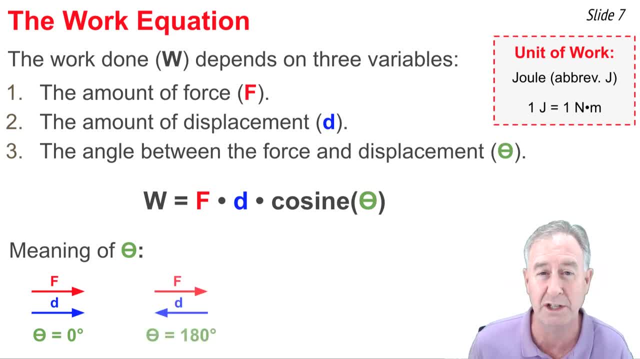 are in opposite directions, then theta is 180 degrees, And if they're neither in the opposite or in the same direction, we simply measure the angle between the force and the displacement vectors, and that angle measurement gives us the measurement of theta in the work equation. 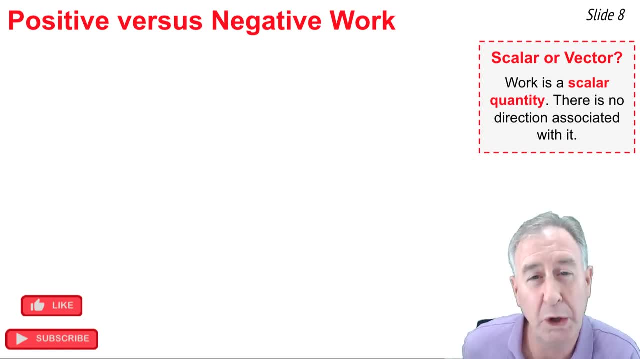 So let's look at the work equation. Let's look at the work equation. In physics, there are scalar and vector quantities. Work is a scalar quantity, that is, it doesn't have a direction associated with it. For vector quantities, like force and acceleration, they 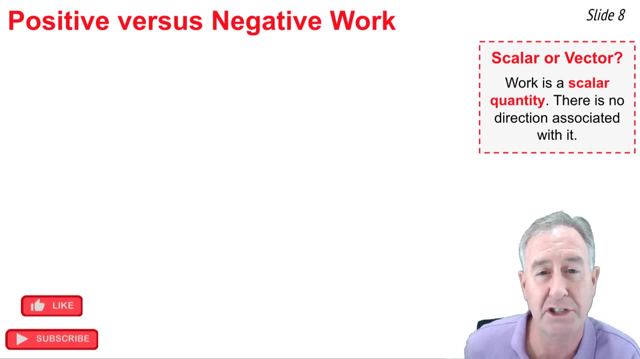 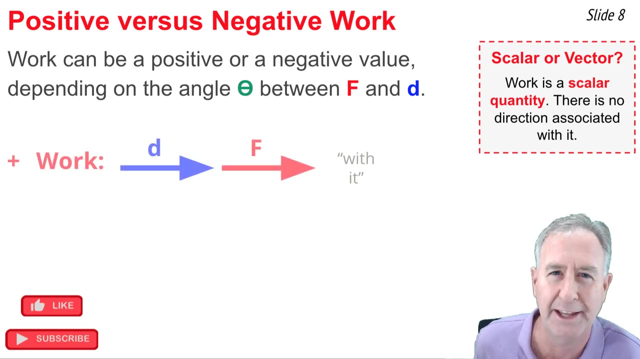 can sometimes be positive or negative, and the positive or negative tells us something about the direction of those vectors, but not so for work, since work is a scalar quantity. Work can be positive or negative depending on the relative direction of the force and the 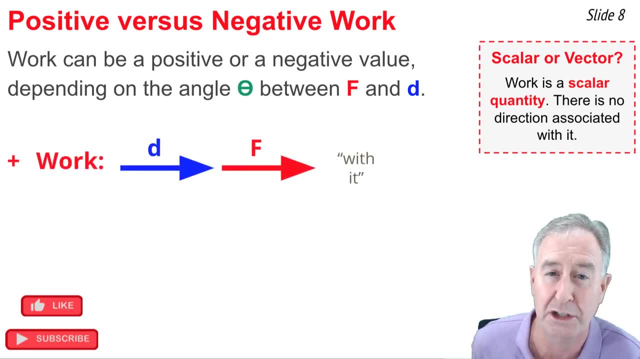 steak. If the work is positive, then work is positive, as opposed to work Plus minus, minus, plus comes to minus minus. since work is negative, Plus minus, minus, plus comes to minus minus, so it is not positive. Then there's the absolute constant. 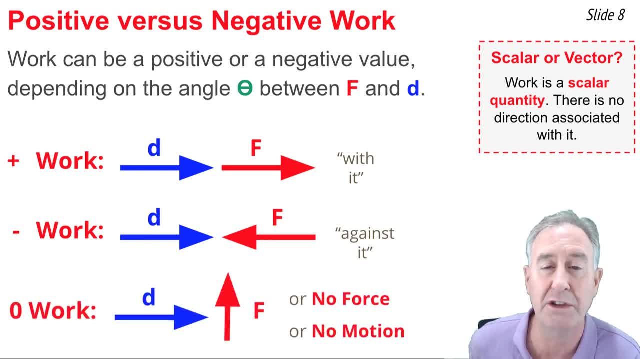 But what about value one? So if value one? so that is, we calculate when the force is diagnosed with its positive einequalts of solve. instead of that, the force is positive or non-negative. the force is talking about the forces that hold greater importance to.